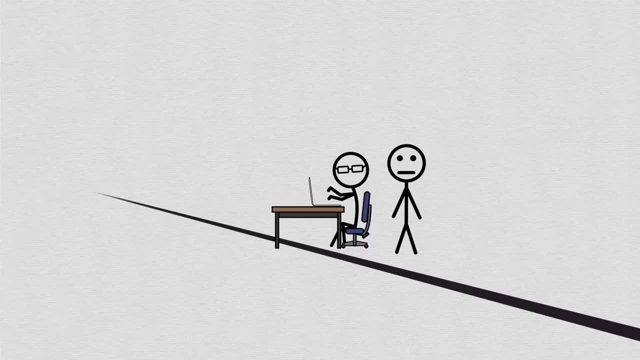 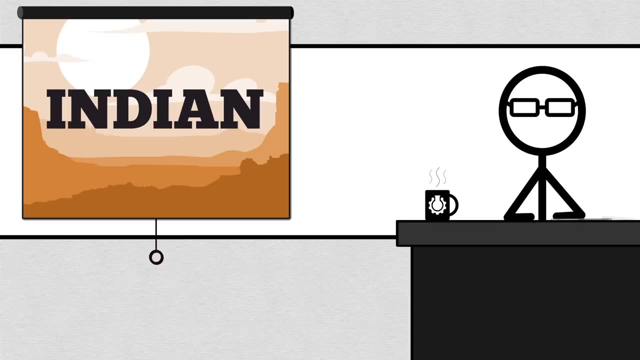 for the first people, Indians. We are in the future from this past and you in the future from my present, possibly the far future, And the word Indian may have just made you uncomfortable. So let's talk about words. Words are what we make them. Without the words, 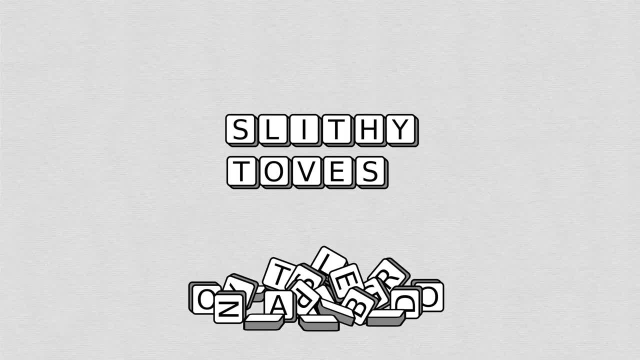 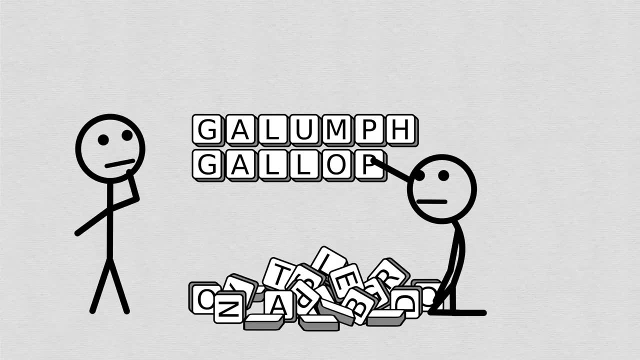 surrounding them. without brains to interpret them, words are but whispers of wind. It's a word's utility to the speaker and the reaction of the listener that causes words to be born and to live and to die, Long after its first use in the New World. 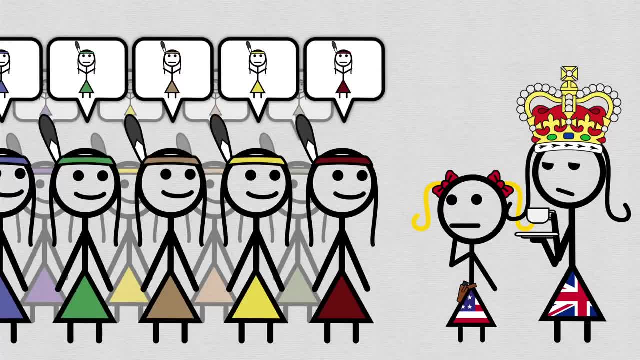 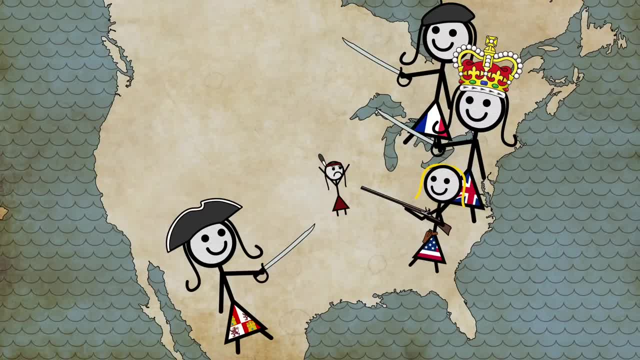 the early British and American empires needed a word to collectively describe the first people, and Indian, despite its confused origins, was that word. As the empires expanded, there was terrible conflict. The first people found themselves decimated and scattered. Many 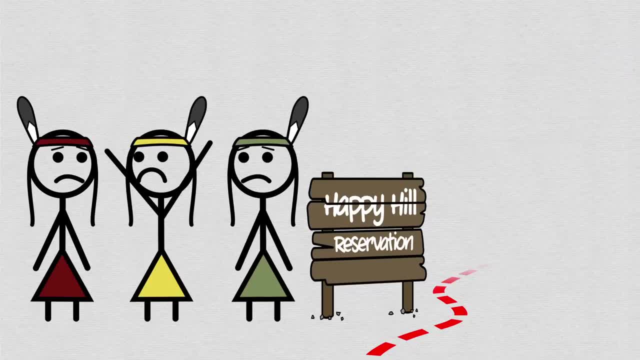 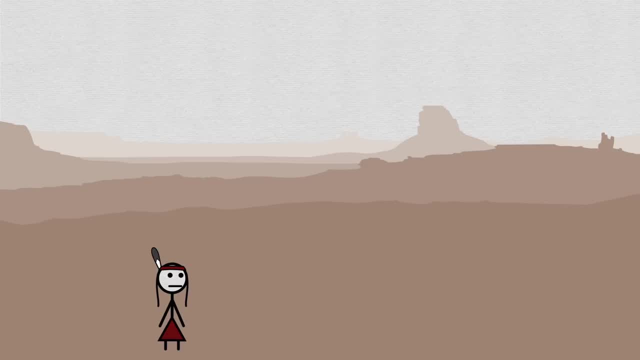 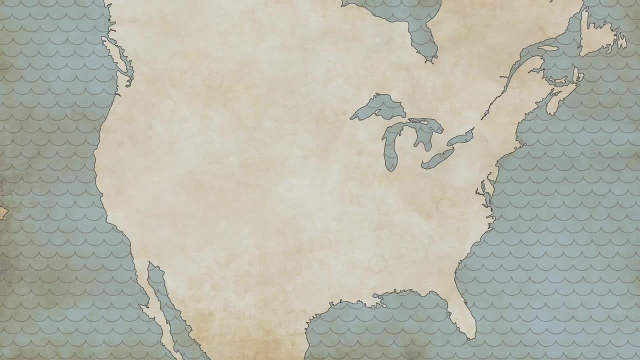 forcibly moved to reservations, land unknown, with others unknown, needing to act as one new group to survive, to hold on to any sovereignty. As the world progressed from horses to steam, to electricity, the nature of conflict changed: Fewer guns and germs, more mines and laws, But the first. 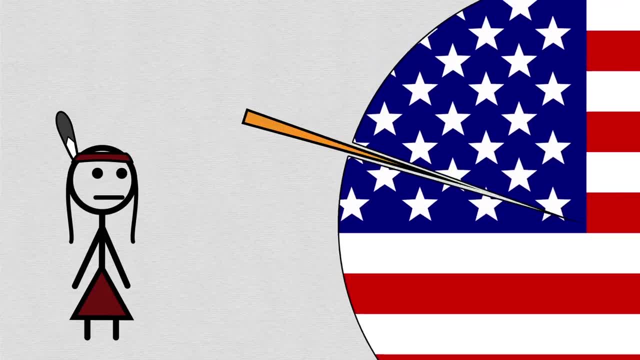 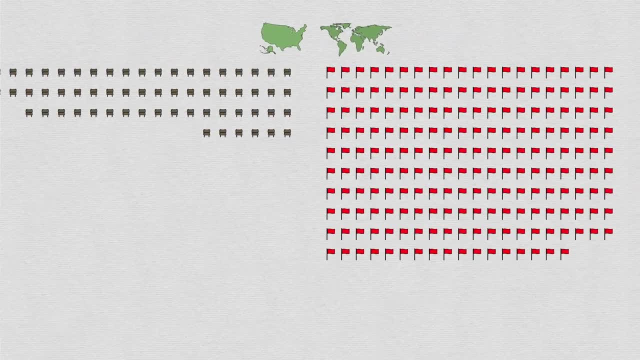 people were now a tiny minority in the land, while also a multiplicity of groups. For comparison, there are about 200 countries in the world. Within the United States, the reservations number more than 300.. Within and without those areas of special sovereignty, there are more than 500 federally recognized tribes, each with a different name. To win the minds of the majority to get laws securing sovereignty, hundreds of different names for different groups is not helpful. A collective name, one clear in the minds of the majority. 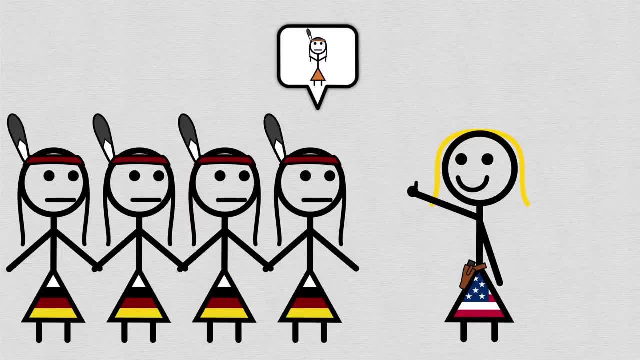 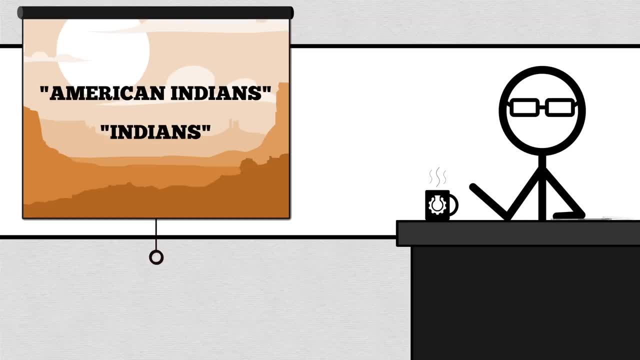 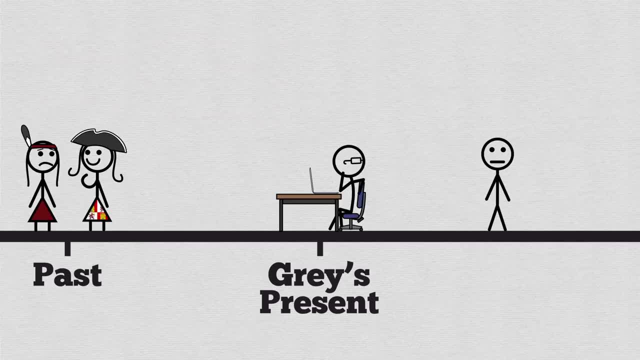 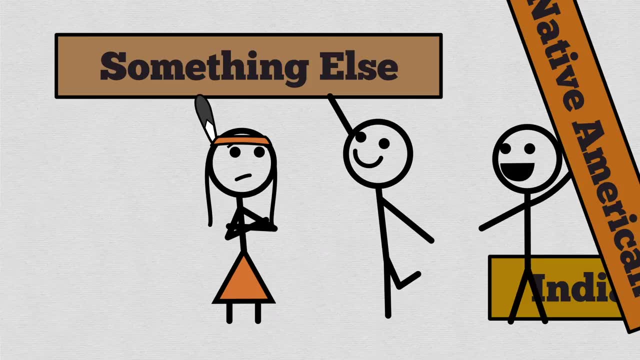 them As I write this script, looking at the past and toward you in the future. I will bet that future history will unmake Indian in favor of Native American or something else. You know if this has happened, But here, as part of working on this series, I've traveled to many reservations to 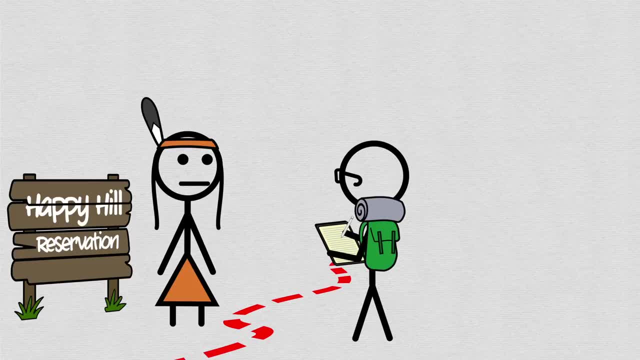 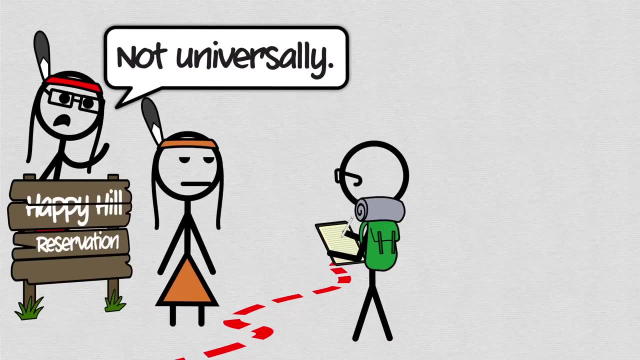 see them and to talk to the people who live in them. On reservations, the word Indian is still used without hesitation or negative connotation, Used as identity, Not universally, but near it. You, like me, are the ones who make them. You are the ones who make them. You are the ones who make them. 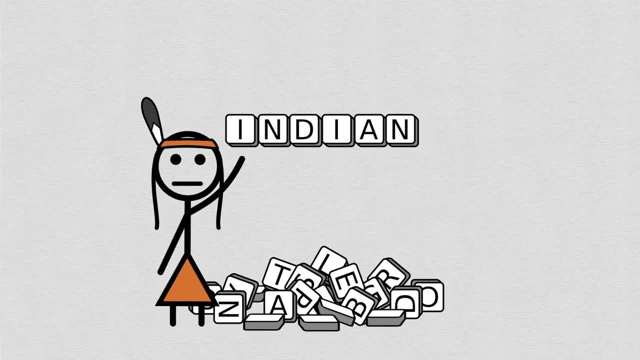 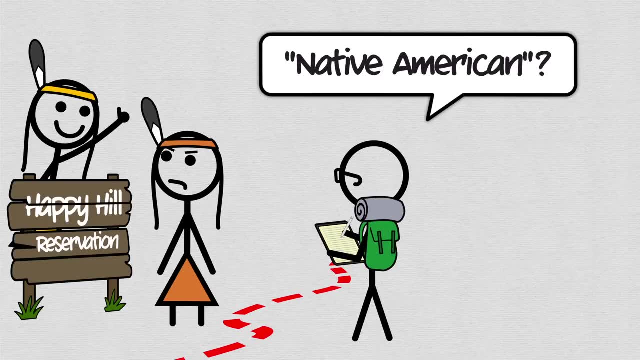 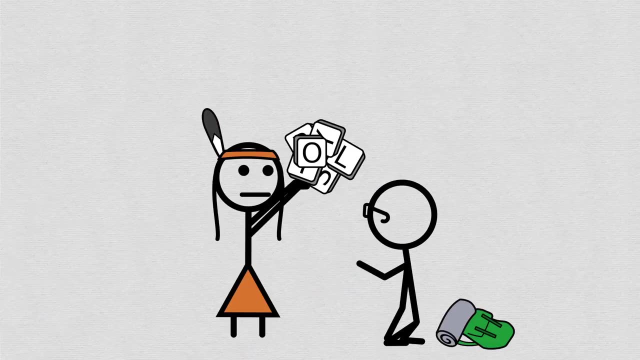 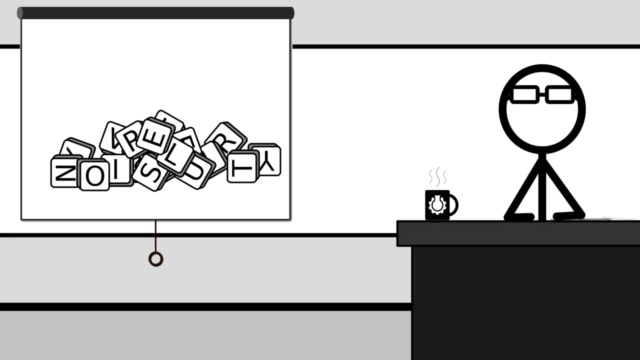 Now, as for Native American, while preferred by some, there exists in others a strong dislike and resentment of the name. The word created to explain this dislike was passed on to me And the only way to explain fully is to pass it on to you. So the dislike comes from over-inclusivity. 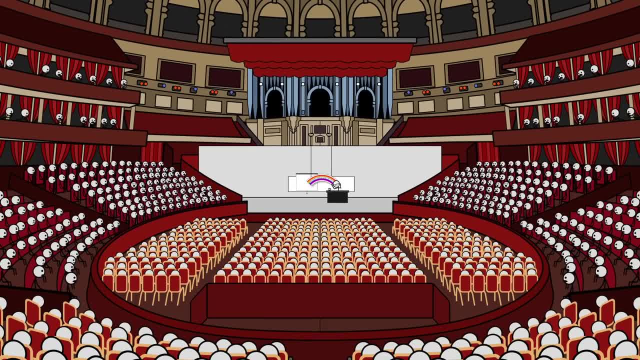 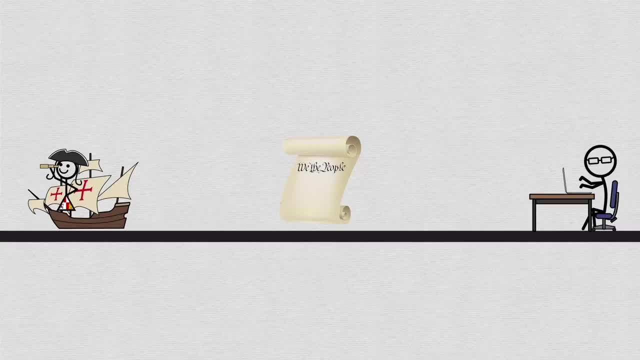 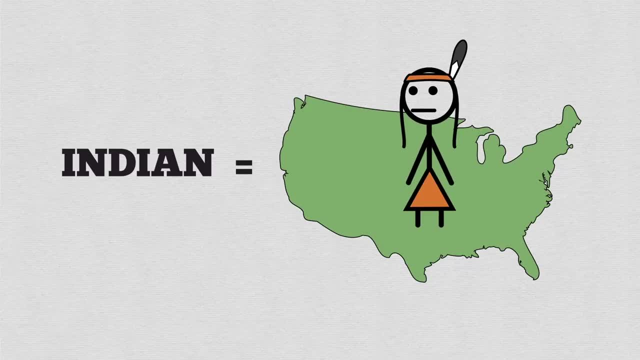 I know, I know, I know, But let's stay thoughtful and examine what this word was created to communicate. For at least 300 years, Indian has meant the first people in this part of the world, separated at first but thrust into a shared history. It is clear, it is sharp, The word. 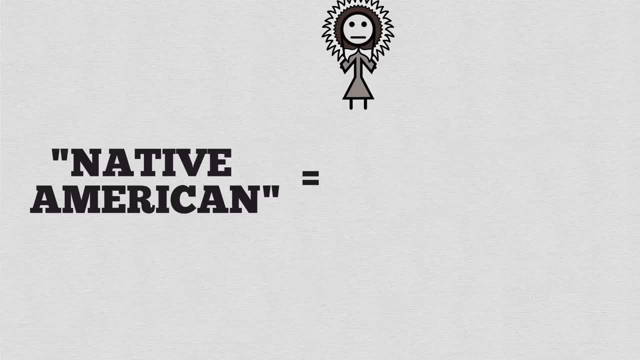 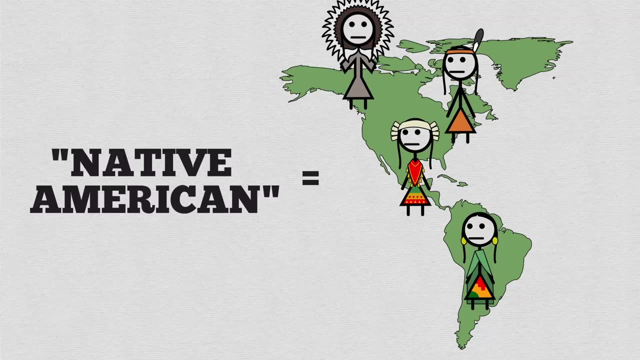 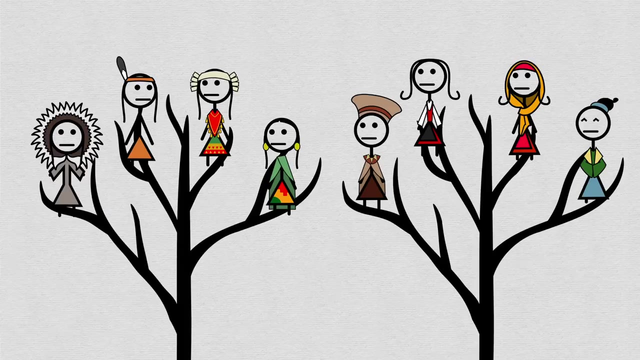 Native American less so. It can include everyone from the top to bottom of two continents, A vast number of different cultures and current nationalities. The history of North, Central and South America are as divergent as the histories of Asia, Europe and Africa. To call a person from here here or here a native Afro-Eurasian would 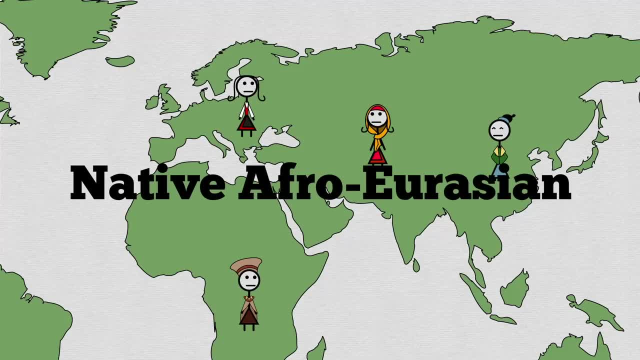 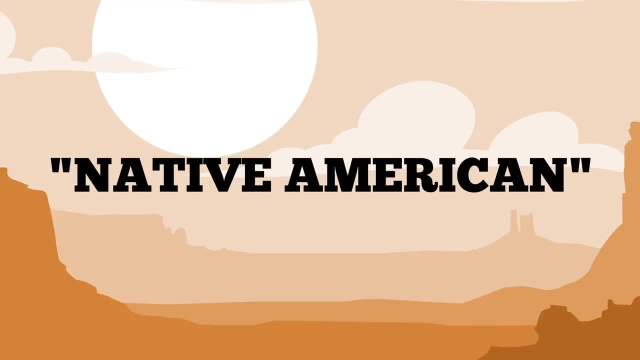 be so over-inclusive as to make it difficult for that human to strongly identify with or rally others under. So it goes for Native American. Additionally, it can feel like yet another thing forced from the outside Talking to people about this project over the last. 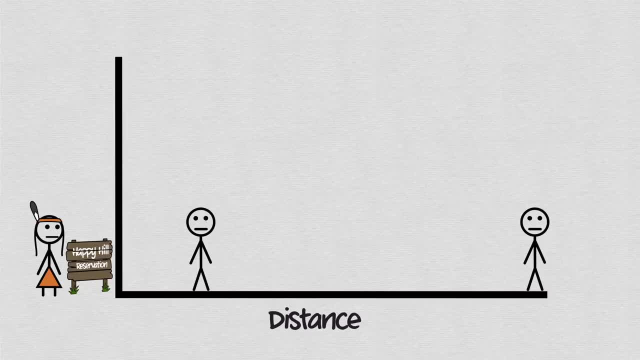 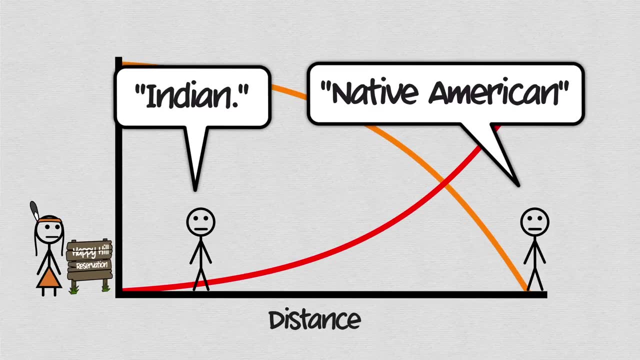 five years revealed a strong correlation: The closer a person had ever been to a reservation, the more likely they would use Indian. The farther, the more likely they would use the word Native American, And that's understandable. Is Indian okay? Maybe, But Native American won't. 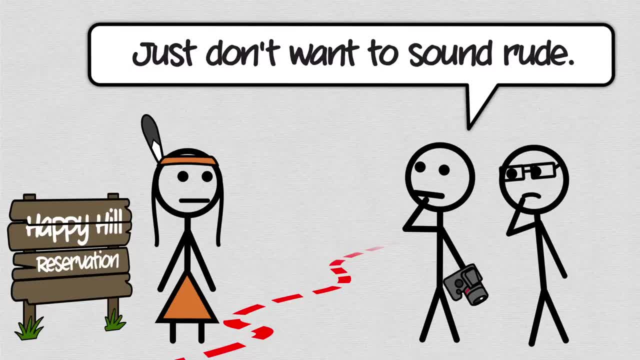 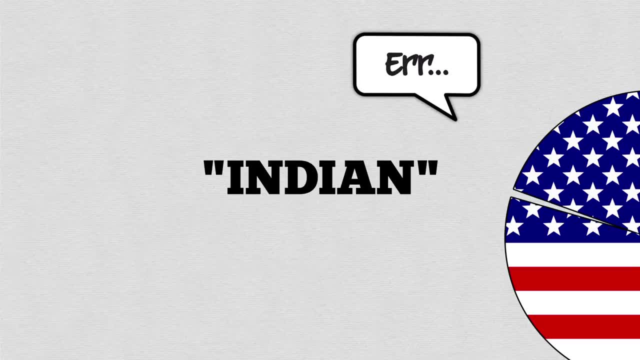 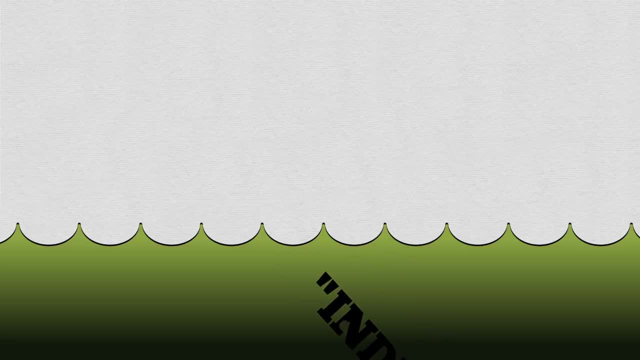 be wrong and it's useful to express concern and sensitivity as an outsider, But this creates an unstable balance between insider and outsider use of a word. If the majority hesitates over a word, it slides into uncomfortability. If the majority decides a word is unacceptable, so it becomes. Groups should be able to name. 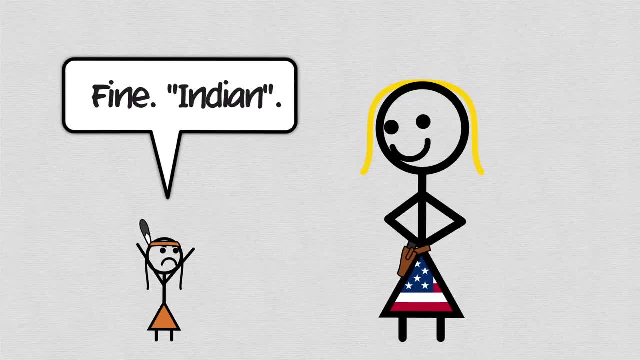 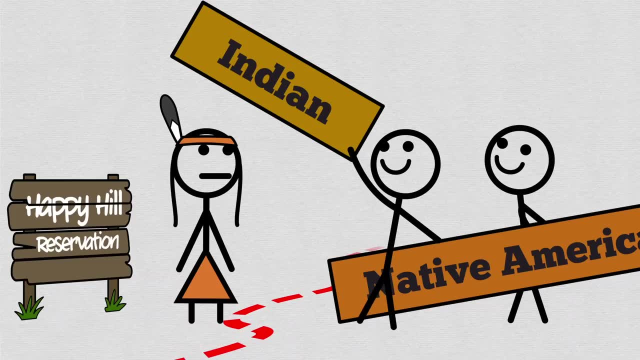 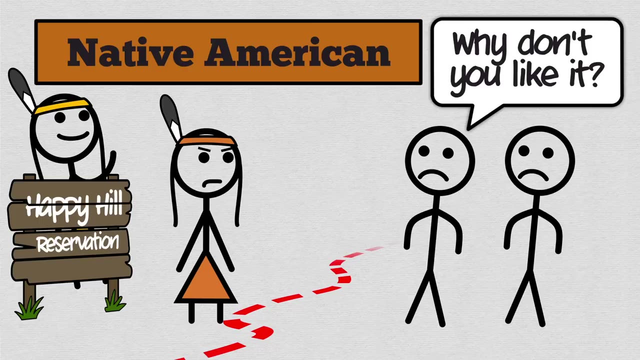 themselves, but when they're small they often can't The word used to describe themselves- outsiders, through sheer numbers, redefine At the time of writing. this is happening to Indian, But the leading replacement is not as universally well regarded inside reservations as those outside may.